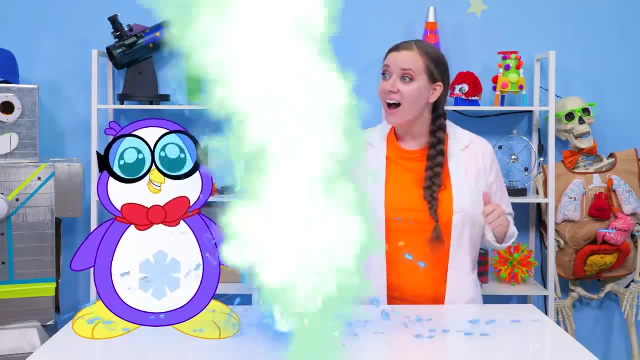 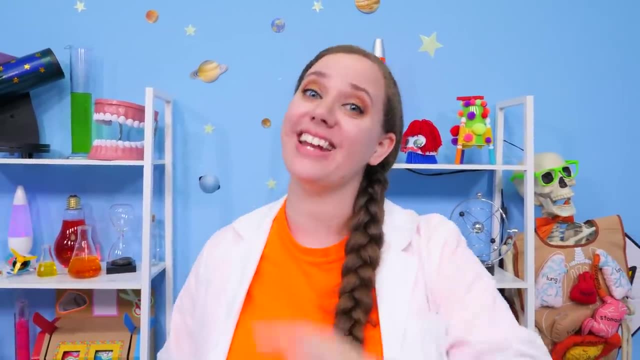 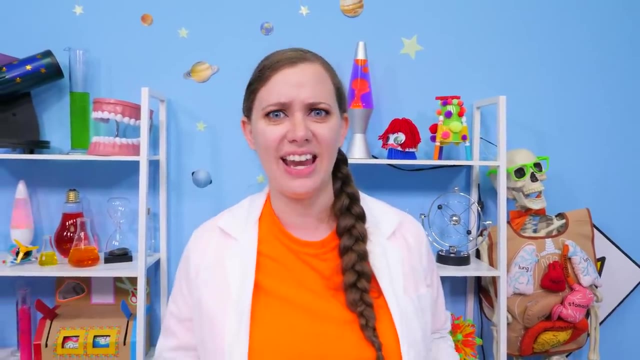 I'm designing a lightning experiment for Ryan Ka-chow. I know We can harness the power of static electricity to build a lightning machine. Excellent, Go ahead and get started. Well, the first step is we need materials, and I'm pretty sure we can find everything around the office, so 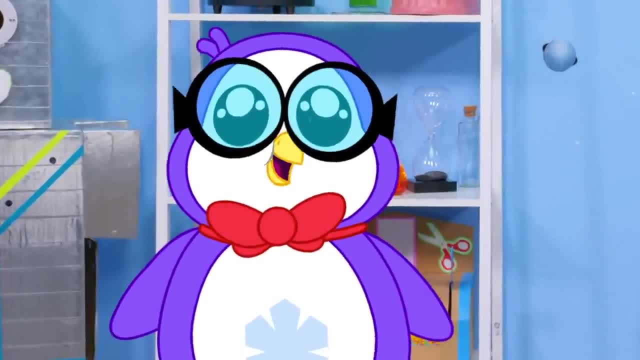 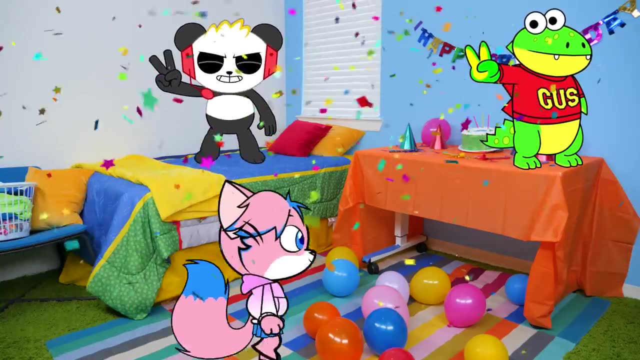 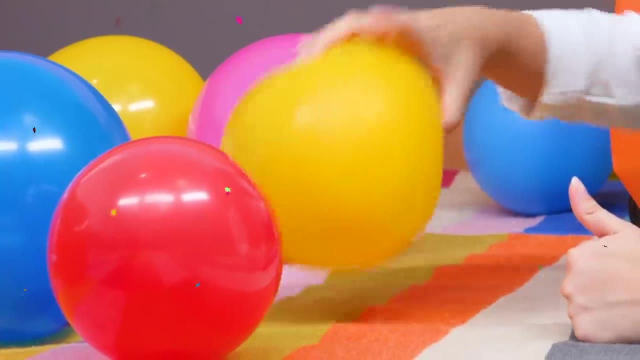 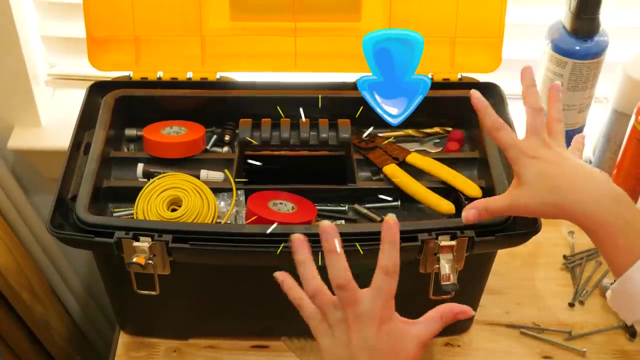 Now I'm going to learn about static electricity after a quick power nap. Hahaha, Woo-hoo, Party time. I want cake. Hmm, I'm ready. Ahem, Well, I have a good idea for a little party party. 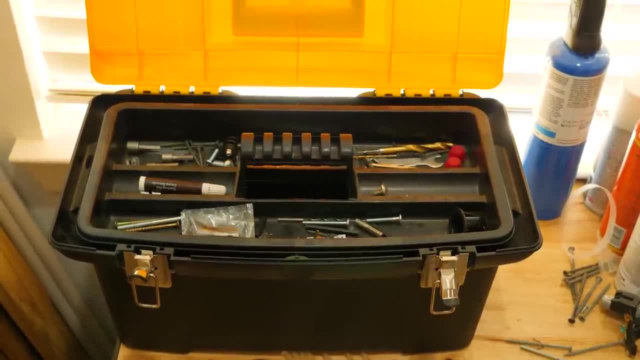 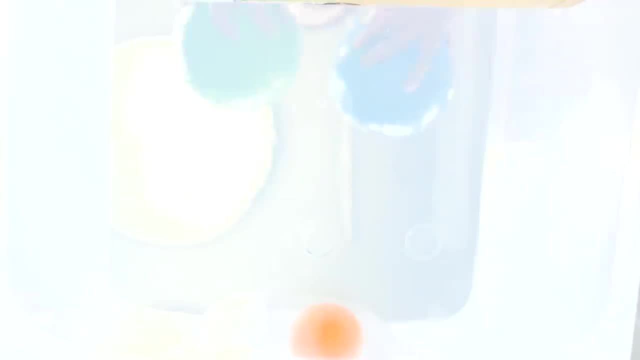 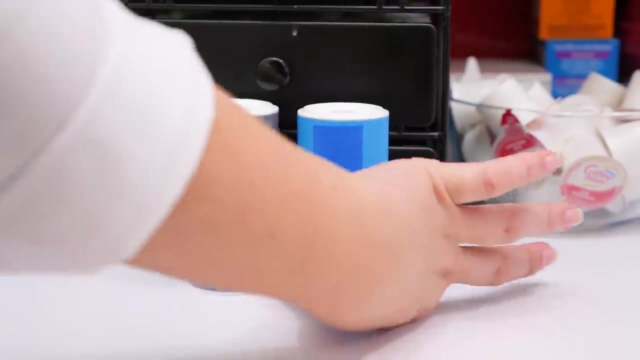 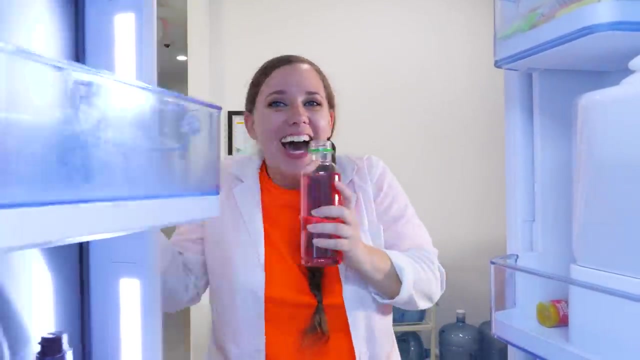 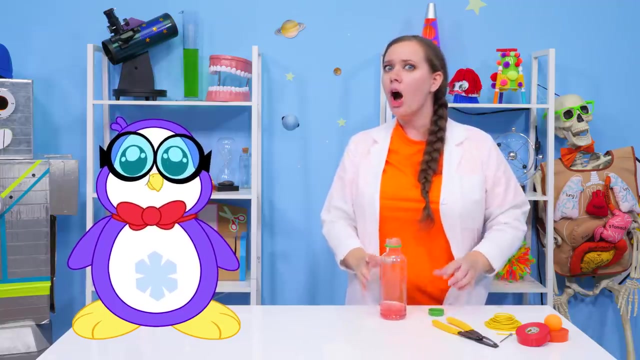 I'll go get some food. Hmm, The sun is about to set. I'm all ready. It is starting to get pretty warm. I'll go get some food. Whoa, did you gather the necessary materials? Oh yeah, um ha got it. 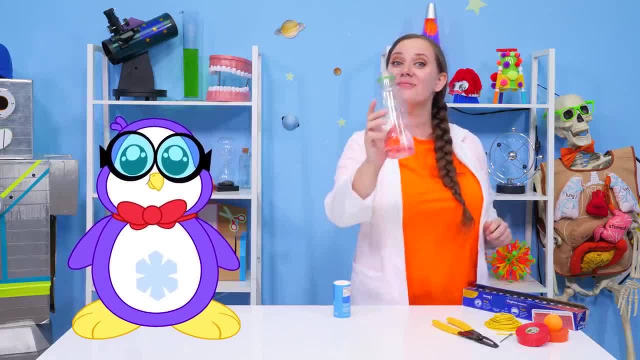 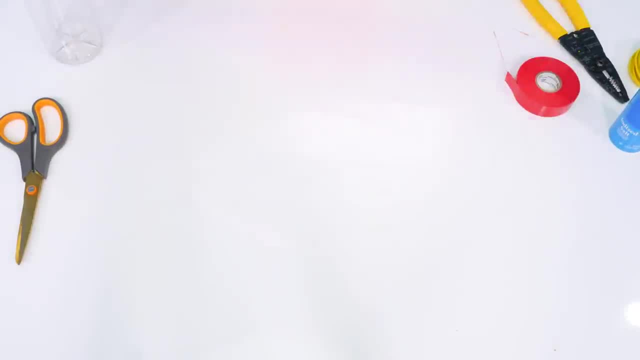 Finish up your drink and let's get started. Sounds good to me. Fancy scene transition For our outside conductor. we're going to use aluminum foil. The first step is to cut our foil to the length of the flat side of the bottle. 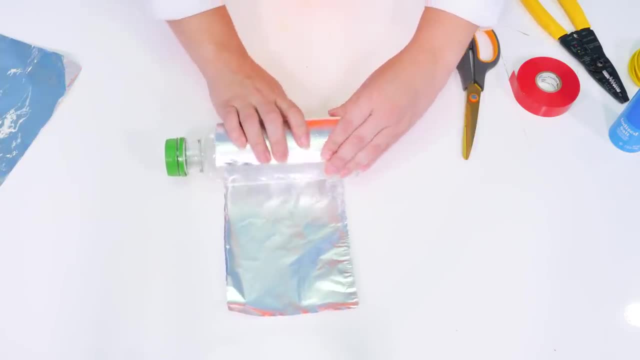 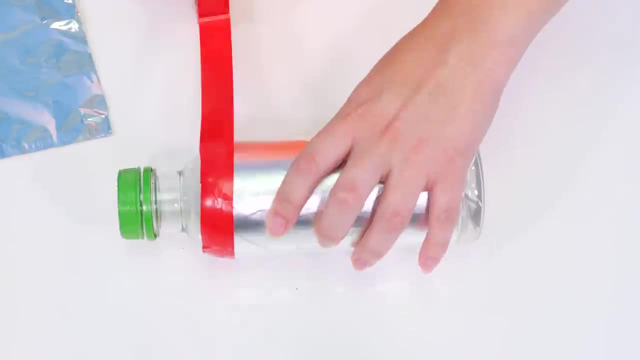 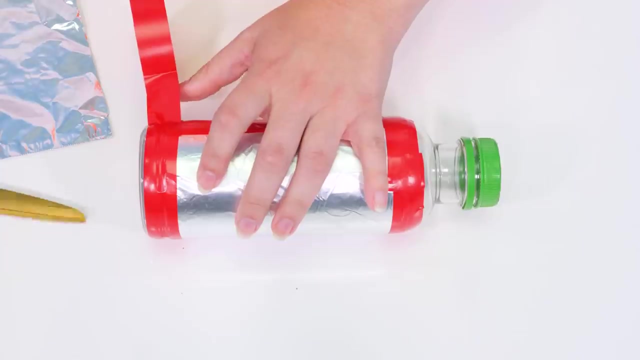 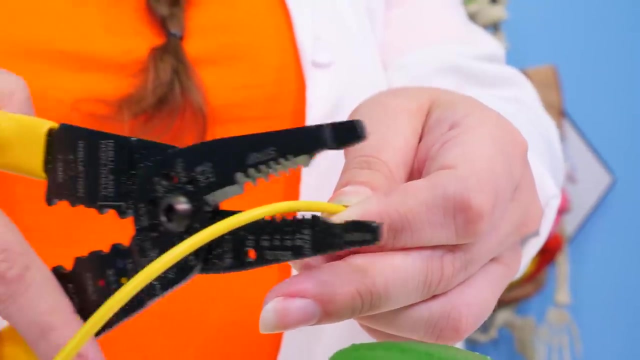 Now that we have it cut, we're going to tightly wrap it all the way around the bottle, making sure it doesn't crease or wrinkle, Then tape it in place and then we're going to secure the top and bottom. Next we're going to measure out our wire to make sure we have plenty of slack, like. 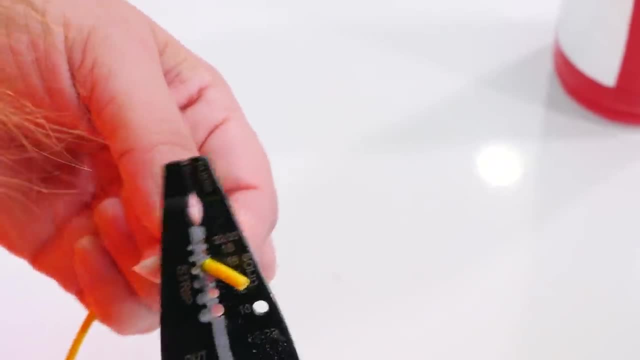 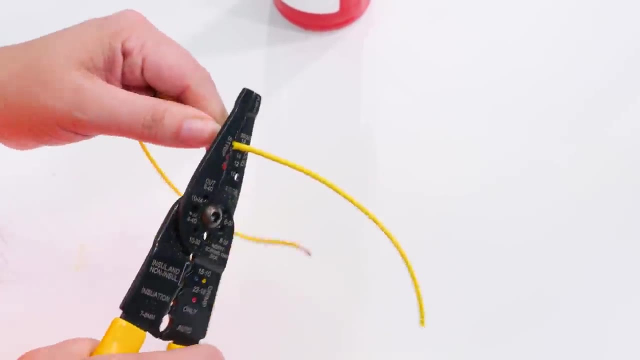 that, Then we're going to cut it and strip off the ends. Now, when using things like wire strippers, make sure to ask an adult for help. The second side of our wire is actually going to make contact with the aluminum foil, so 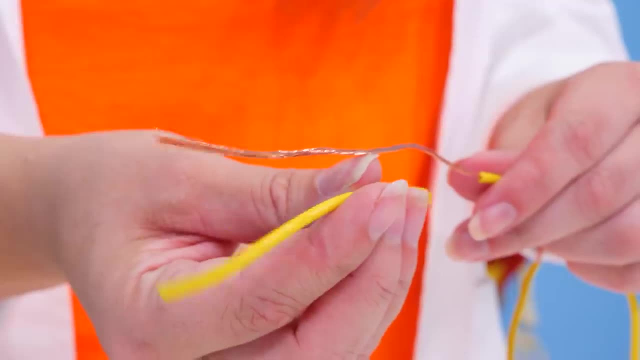 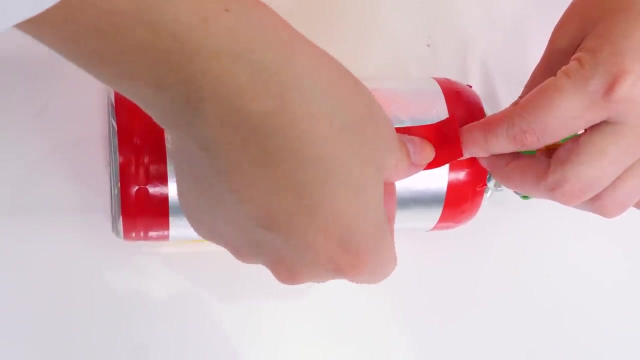 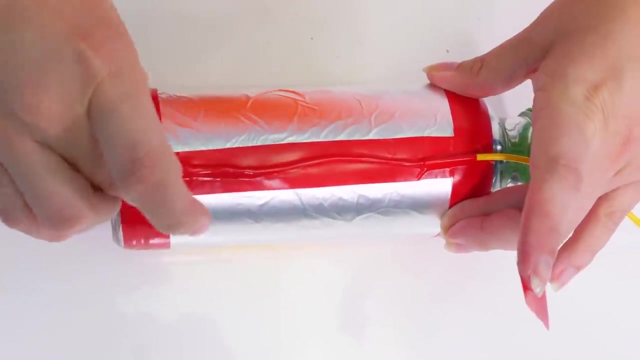 we need to pull off all of that coating like that. Now, very carefully, we're going to lay our wire down and make sure the cotton is in the right place. The upper wire makes good contact with our aluminum foil. Now that it's in place, we're going to tape it nice and secure. 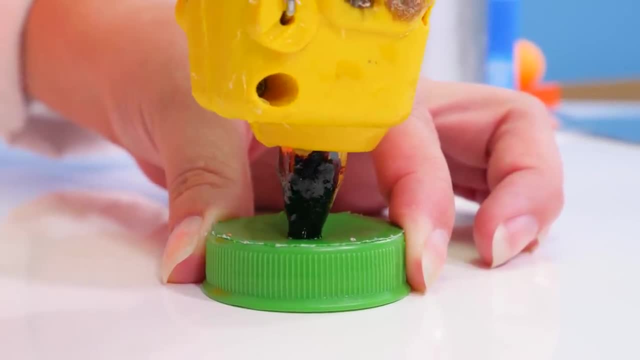 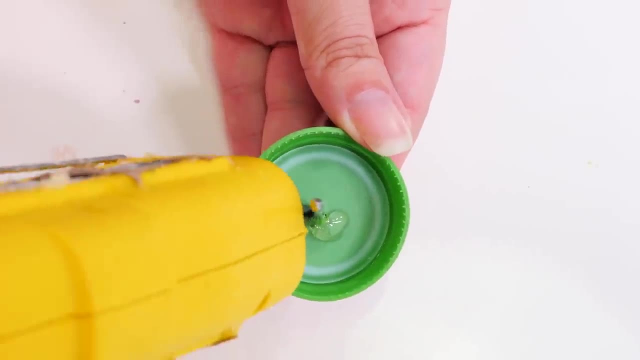 Next, we're going to use the tip of the hot glue gun to melt a hole through our bottle cap. This is going to give us the perfect hole for our nail to slide through. Now we're going to glue it in place. Here it is. 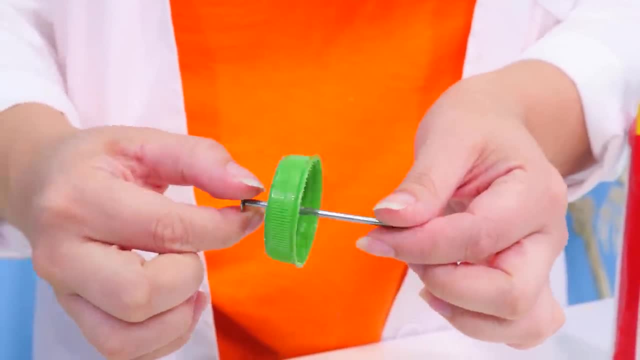 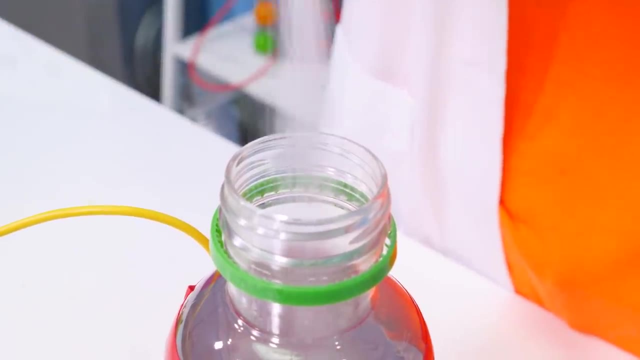 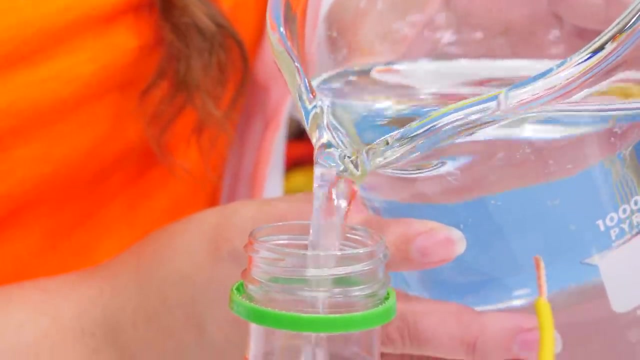 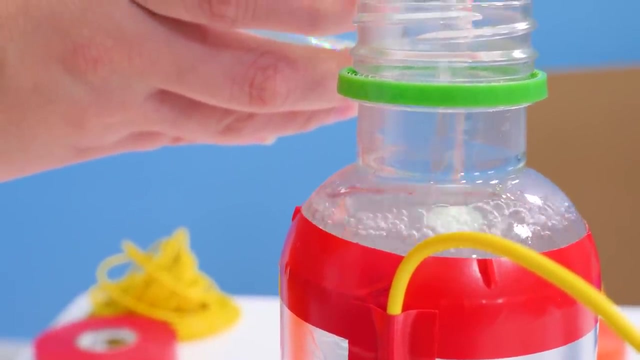 We've got our lid with our nail glued in it, So the next step is we're going to add salt water. Ingredients are simple: It's just salt, lots of salt and water. We're going to fill it up all the way until it gets right past the tape. 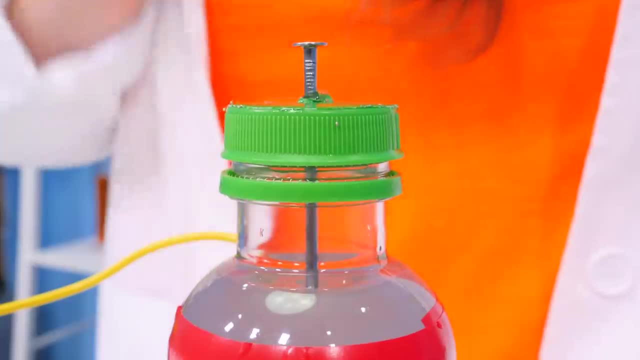 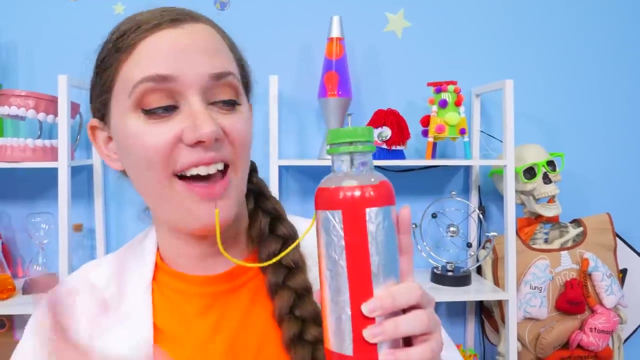 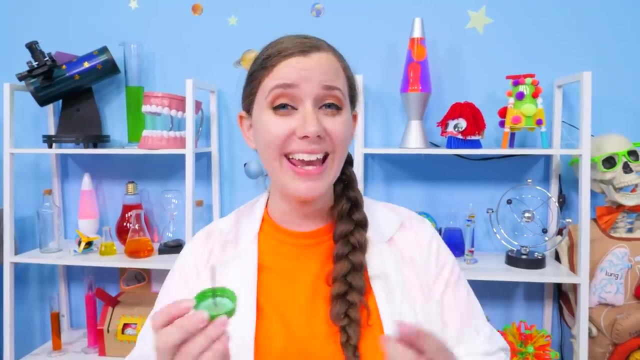 Screw on our lid and shake it up. Perfect. And now we have our salt water made, But the nail is not actually making that much contact with the salt water. What we can do is we can add on more conductive metal to make this longer and give us more. 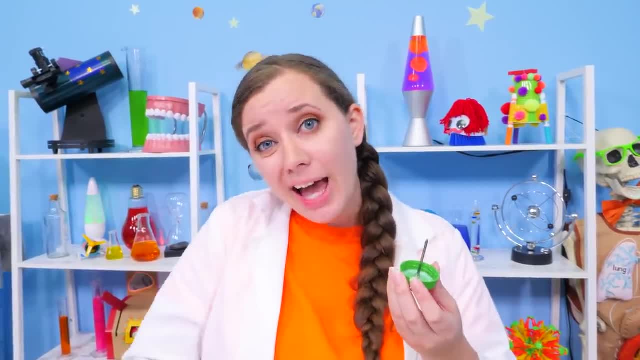 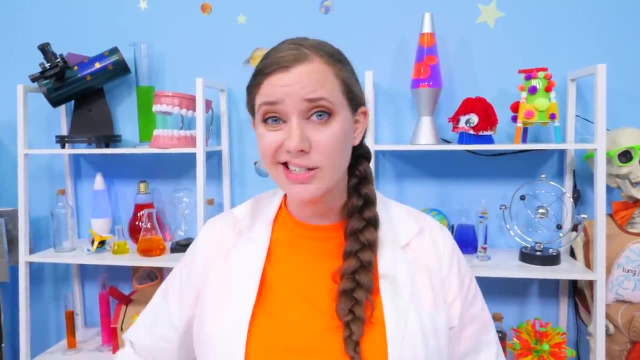 surface area for our salt water to touch. Now, because we're in the lab, I happen to have copper wire lying around. But if you don't have anything like copper wire or maybe a metal chain, you could always just tape some nails together and make it longer. 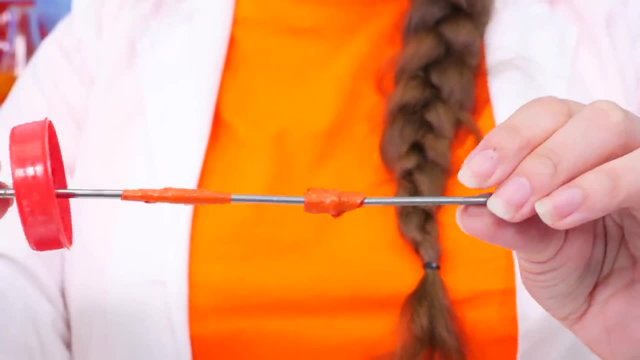 As long as the metal is touching the metal, it'll work just fine. We are going to use our copper wire. We're going to use our copper wire. We're going to use our copper wire and our state-of-the-art pencil to make our coil. 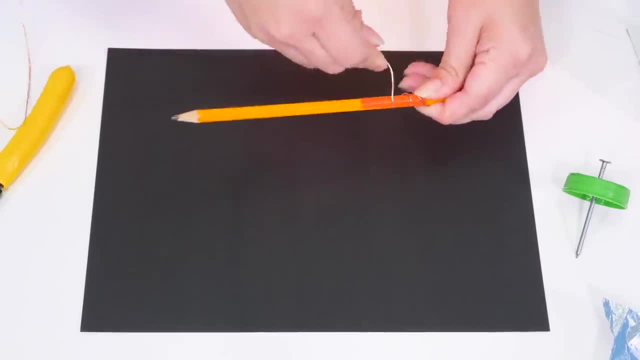 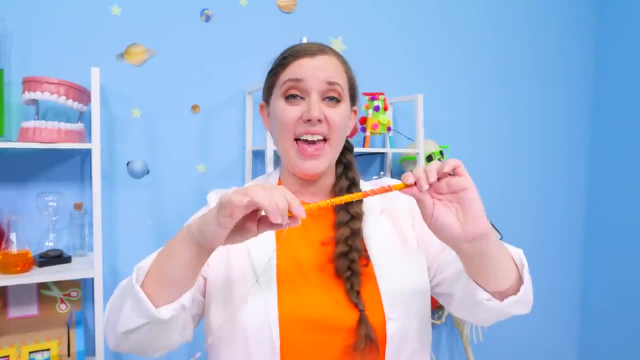 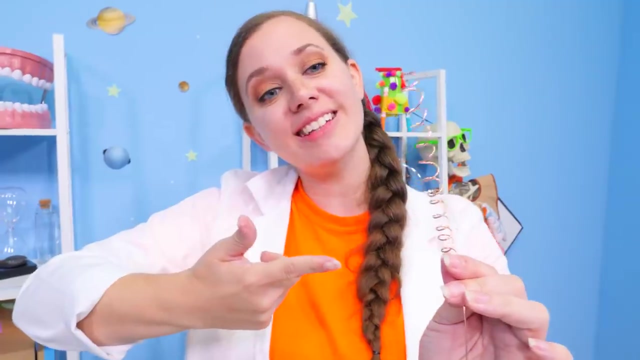 So we're going to start by wrapping around and around, and around and around. but we got smarter, so now we're just rotating the pencil. That's a lot less work. Now that we have it all the way wrapped around, all that's left is to slide it off and boom. 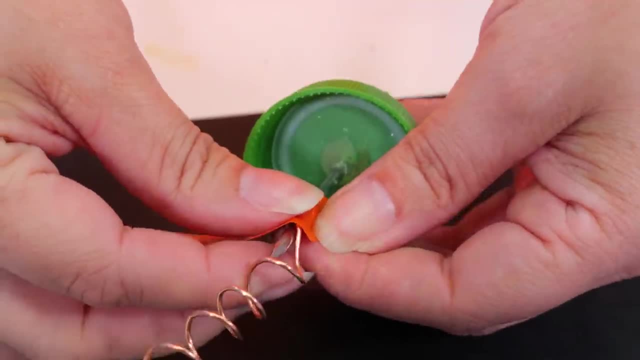 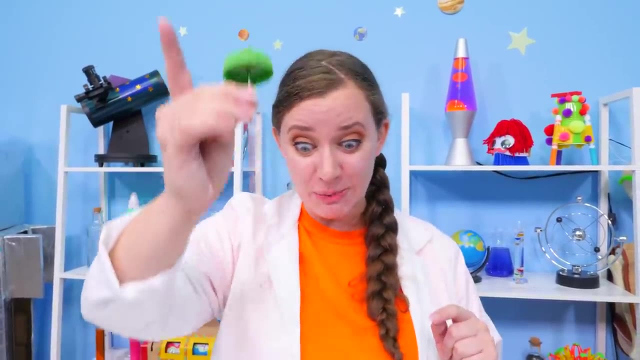 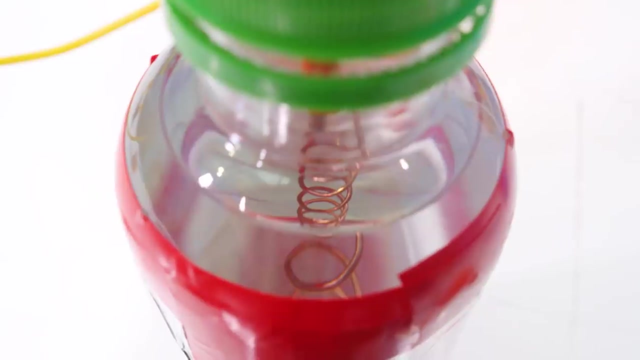 coil. We're going to tightly wrap our coil around the nail and secure it into place with some tape. And now it's time to add our coil to our experiment. Whoa, And now we're making a lot more contact with our water to conduct electricity. 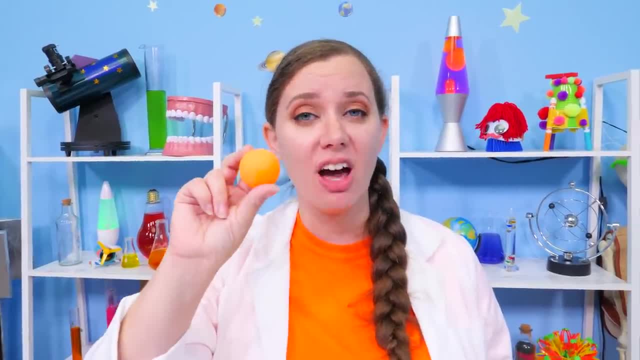 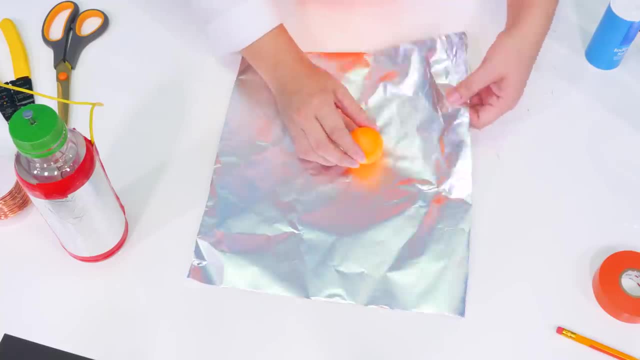 Now all that's left on our build is to add the ping pong ball on top, but since we need it to conduct electricity, we're going to wrap it in aluminum foil. We need to cover the entire ball with aluminum foil and get it as smooth as possible. 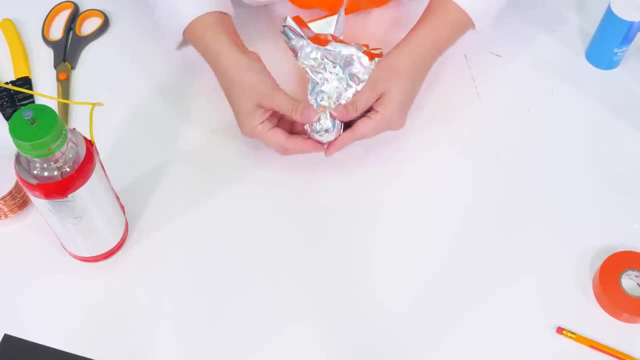 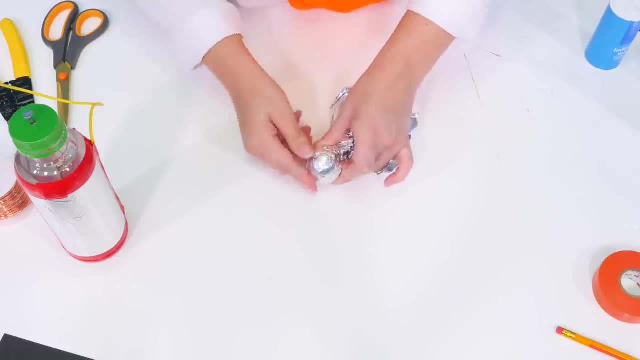 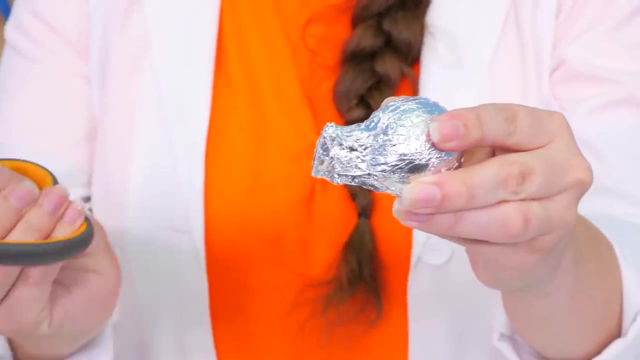 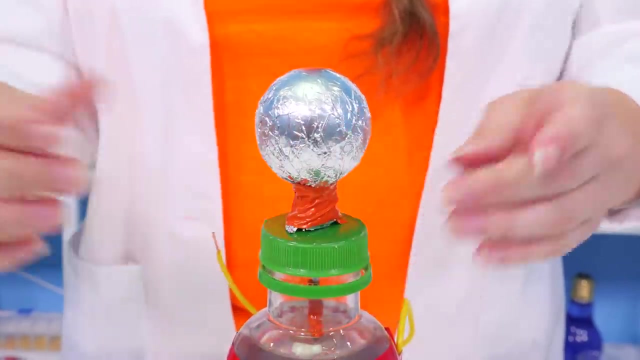 When trimming our aluminum foil, we need to make sure that we have enough extra to go around the top of the nail. Then we're going to smush it into place and secure it with tape Like that. Now we're finished with our build, which means the next step is to charge it up. 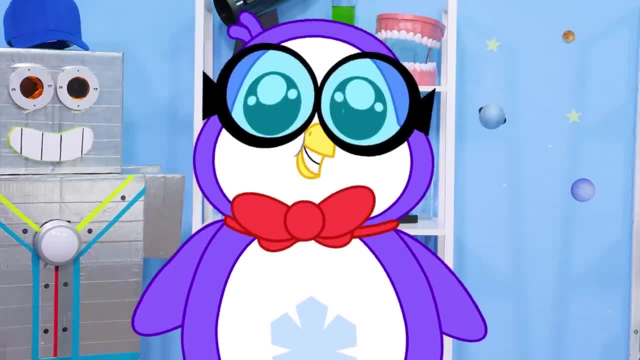 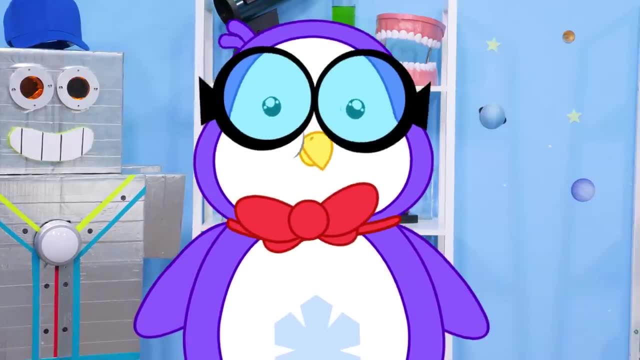 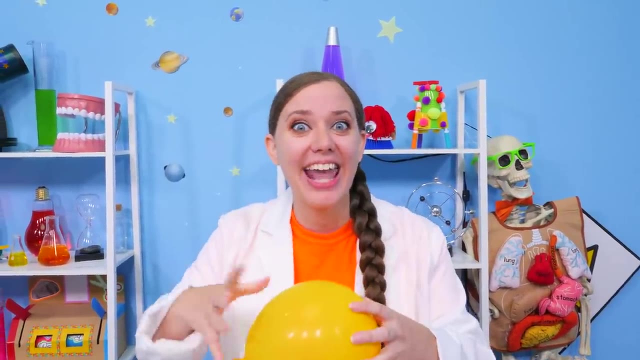 Oh gosh, Are you going to charge it without batteries? Oh man, Oh, that's simple. We are going to use this balloon. Wait huh, How is a balloon going to charge it? Well, we're going to use this balloon to generate static electricity, like this: 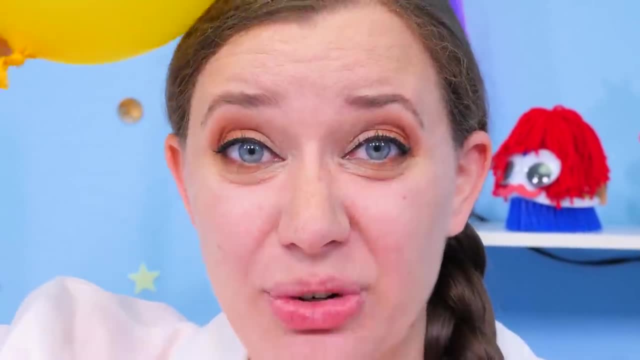 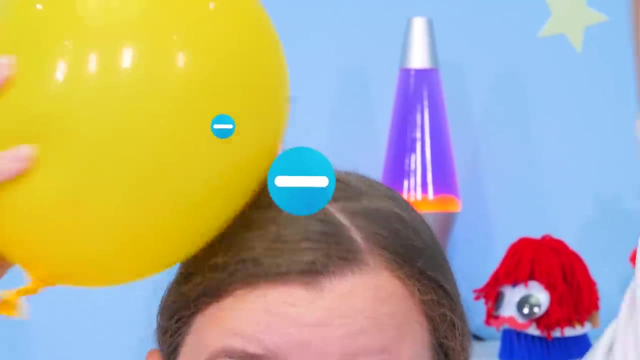 Oh, static. Static electricity is generated when two surfaces are rubbing together like this. Now, in this case, electrons are transferring from my head onto the balloon. Now, because it has more electrons, the balloon becomes negative and my head becomes positive. 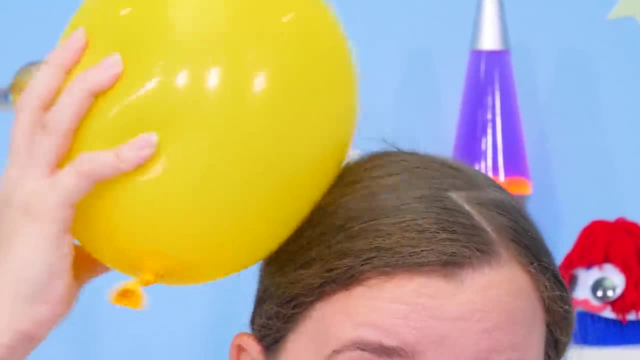 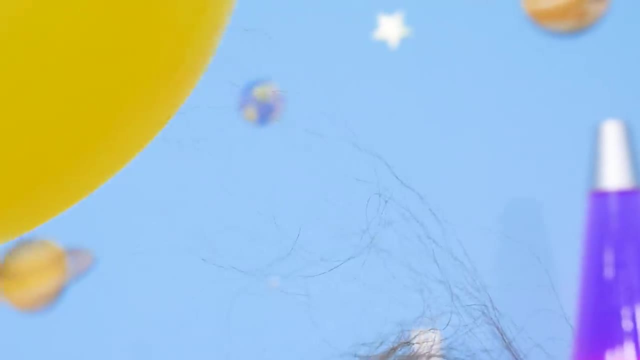 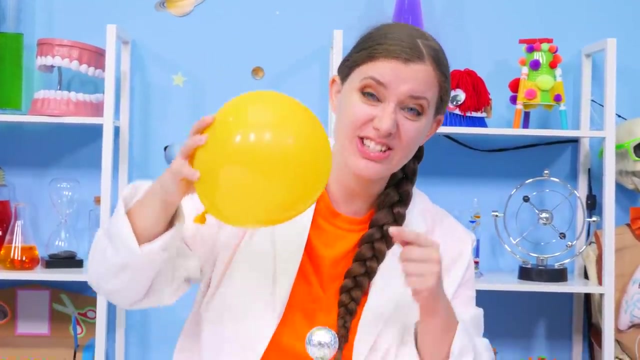 which, as you know, opposites attract. So when you lift it, the hair is attracted to the balloon. Look at that hair go. Now that the balloon holds a negative charge, we're going to transfer our negative charge to the inside of our bottle, like that. 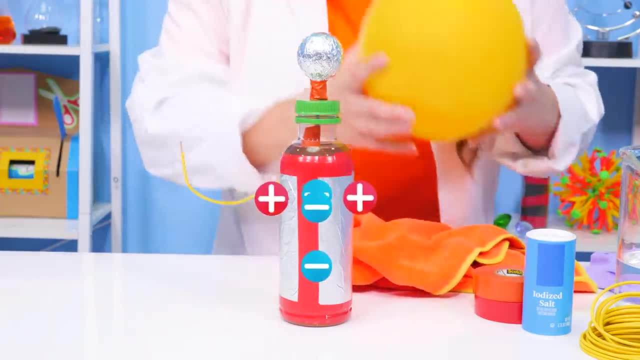 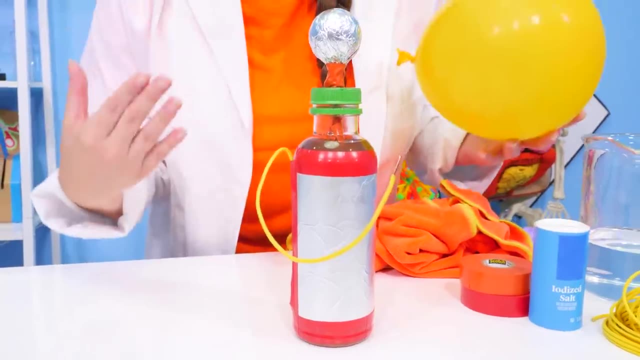 Now the inside of our bottle holds a negative charge, which is actually going to push electrons away from the outside of our bottle, and so the outside of our bottle is now positive, But because things like to be neutral, we are going to use this wire to connect the two charges together. 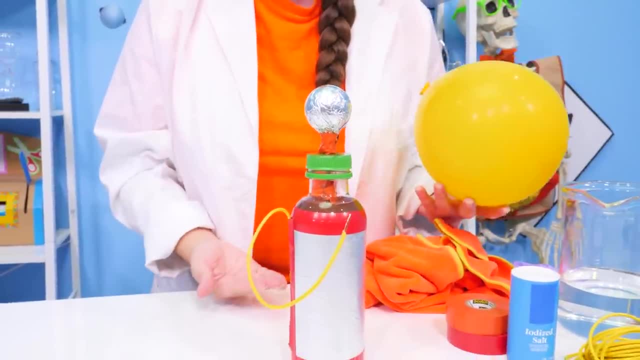 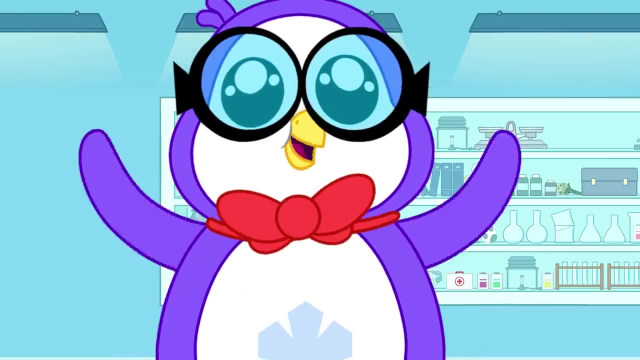 which will neutralize both the inside and the outside of the bottle. In order to charge it, we need a lot more charge. Whoa, This is just like how lightning forms. Clouds are made up of water droplets and ice cubes. 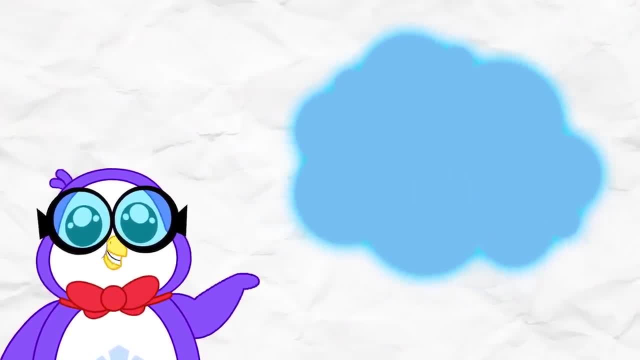 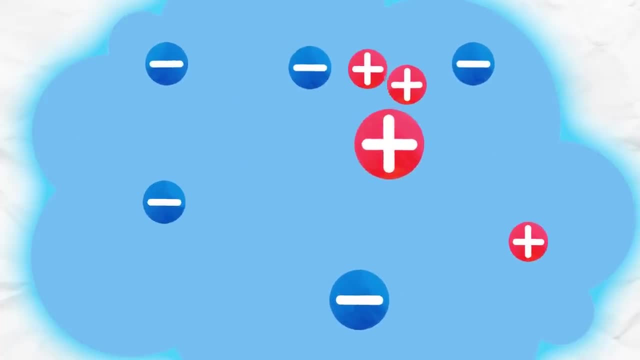 They all hold an electrical charge, both positive and negative. As these particles move around in the clouds, they rub together. The friction causes the positive and negative charges to separate, which creates the static electrical charge. The top of the cloud becomes positively charged and the bottom becomes negatively charged. 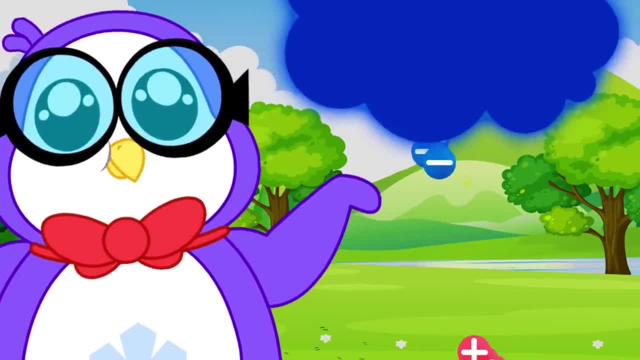 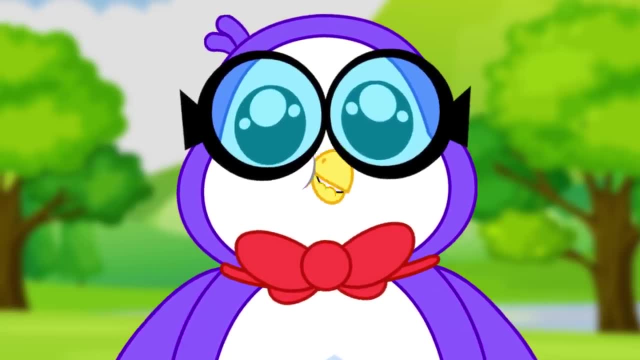 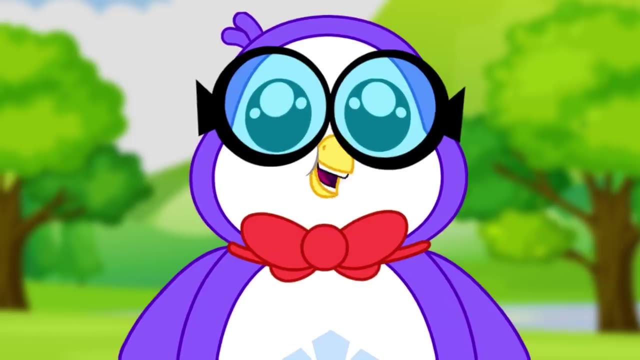 Because opposites attract. the negative charge of the clouds want to join the positive charge. But it's really difficult for electricity to move through the air. As the clouds continue to grow, the charges get more and more powerful. Eventually the charge in the clouds is strong enough to release. 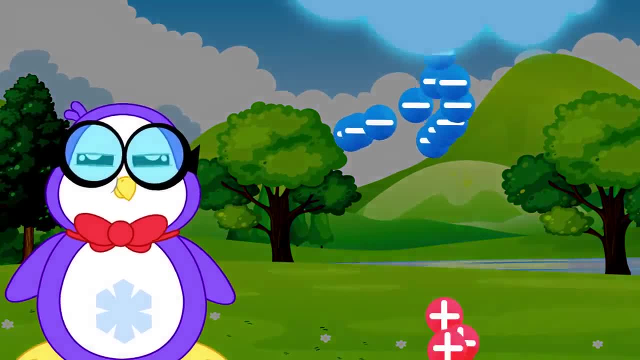 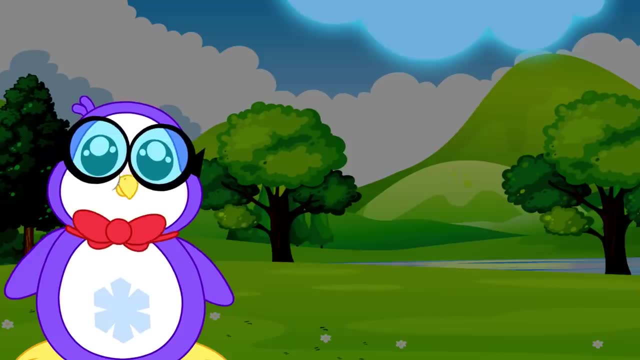 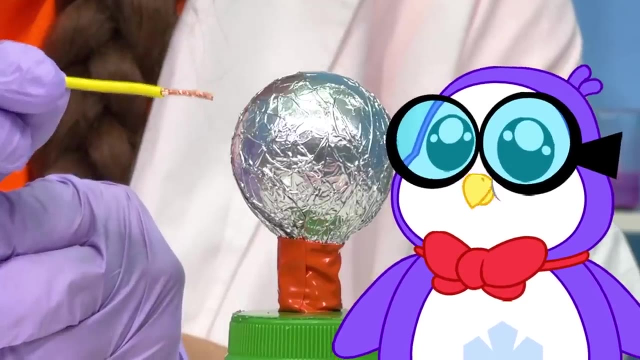 The positive charge in the ground will jump up to meet it and, as the currents join, they create a bright flash known as a lightning flash. This is the same lightning flash that we will see between our water bottles. The lightning flash will be a fire and ping pong ball once the experiment is charged. 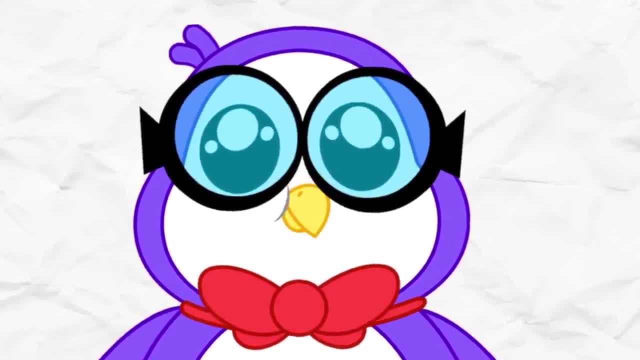 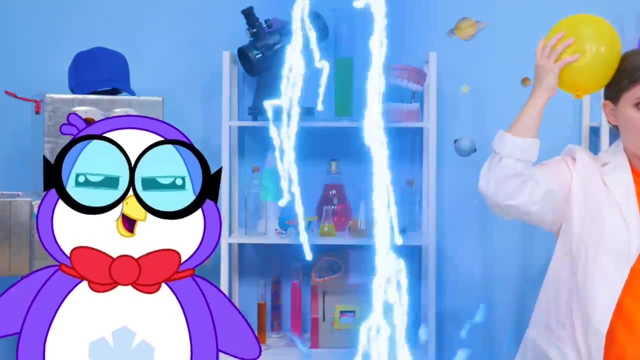 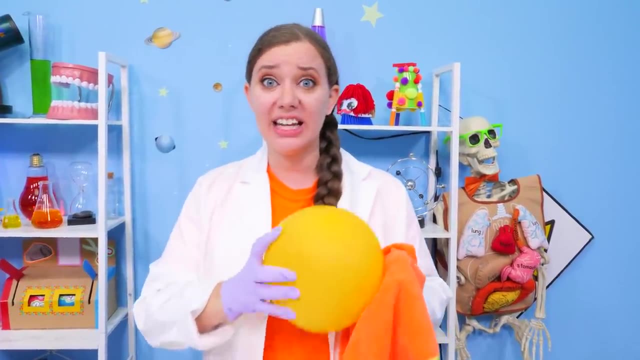 Static electricity is forming around us all the time, like socks rubbing on the carpet, a small shock from a door handle and, of course, lightning. That's exactly right Peck. My head started getting a little tired, so I've been using this towel that we found to generate static electricity. 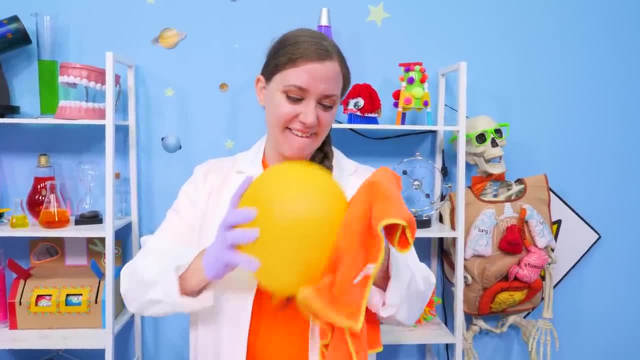 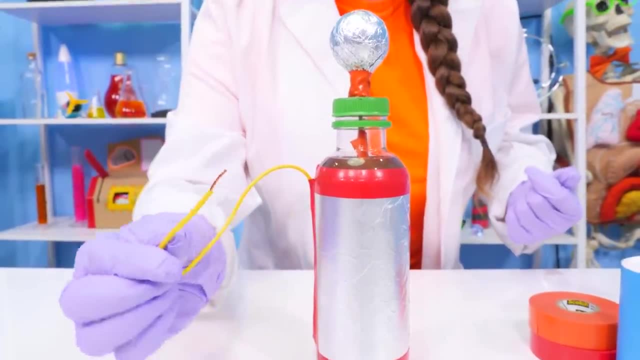 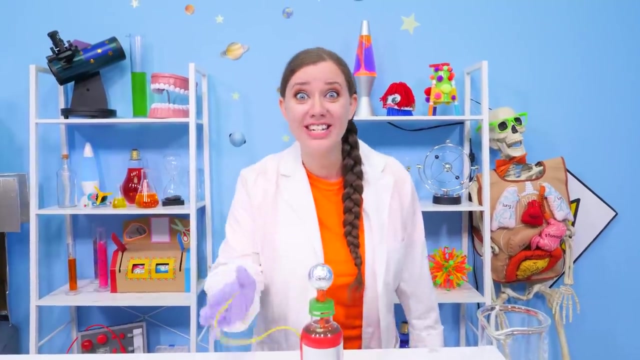 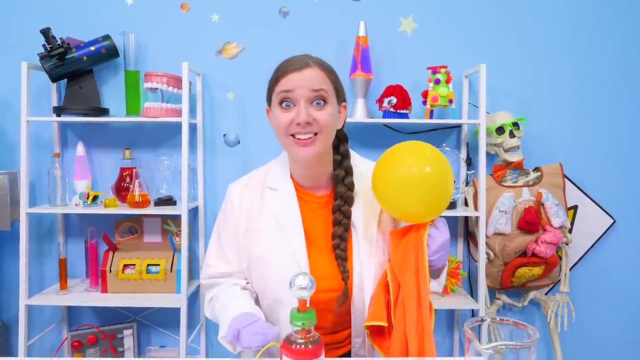 and it's working great. One more charge- Perfect. Now I think it's ready to test. Whoa, did you see that That was so cool? Now, with this experiment, the more you charge it up, the bigger the spark is going to be. 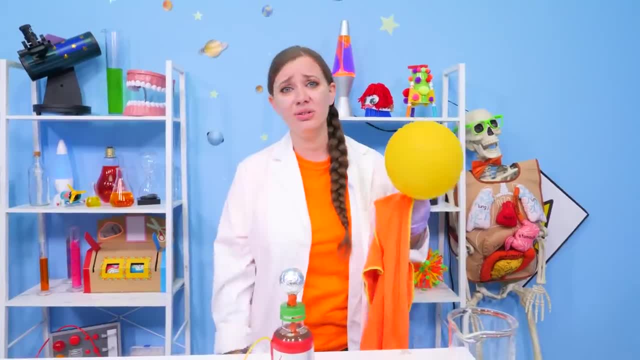 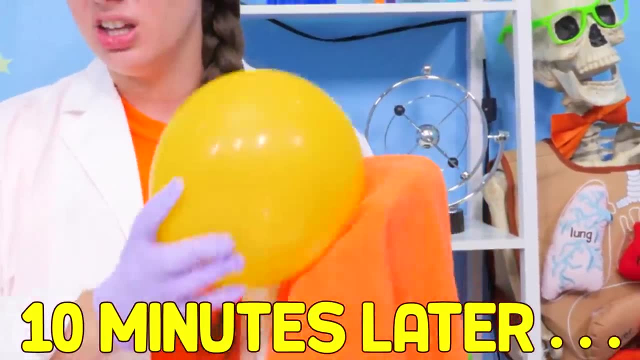 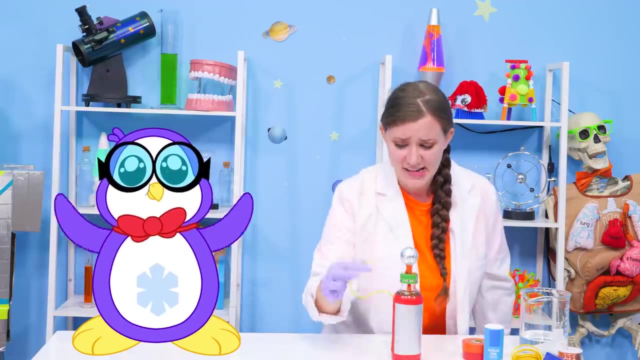 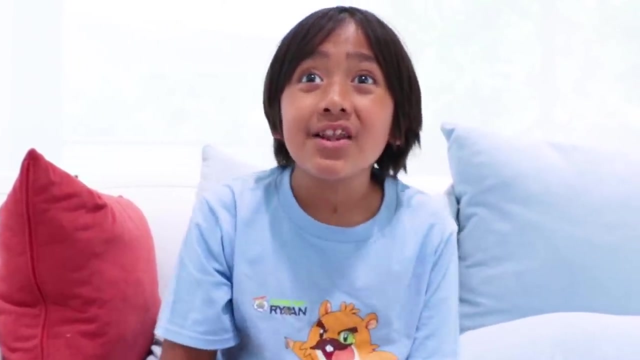 Let's go for a super spark. Okay, but this is going to take a while. Ten minutes later, Ninety-nine One hundred, All right, Whoa, that looks so cool. It's a lightning in a bottle. Peck, you inspire me.